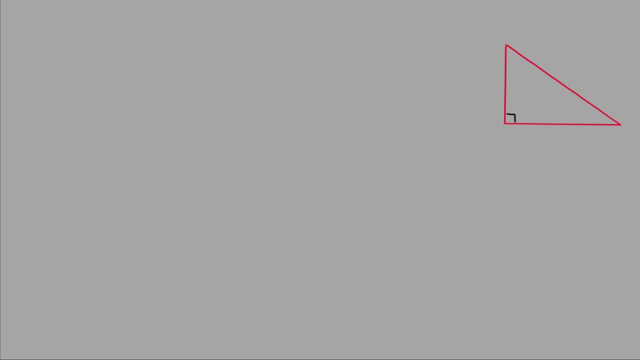 Before we can perform any trigonometric function, we must first know a little about the triangle we're working with. Trigonometry only works with right triangles. A right triangle must have a 90 degree angle, symbolized by the little square right here, Because we have a right. 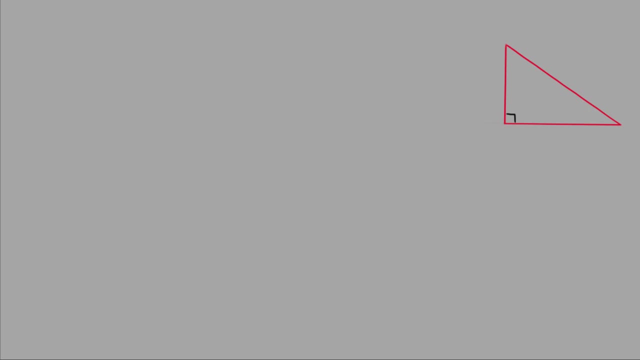 triangle. we can do trigonometry. It is important to know how to correctly identify the sides of the triangle. The longest side of the triangle is called the hypotenuse. The hypotenuse is always going to be the side that is directly across from the 90 degree angle. So if you 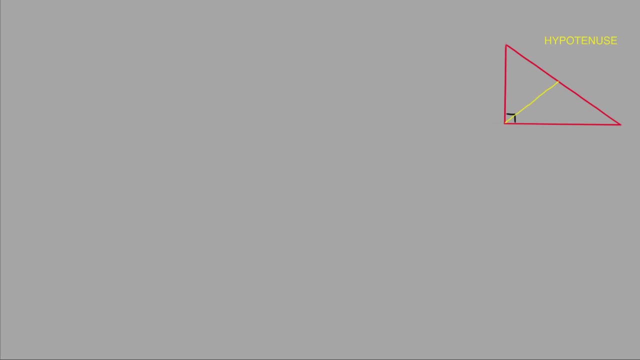 draw a straight line out from the 90 degree angle, you will intercept with the hypotenuse. The other two sides of the right triangle are relative to theta. Theta is a variable used in trigonometry to represent an unknown angle. If I place theta on this angle here, that would make this side the opposite side, The. 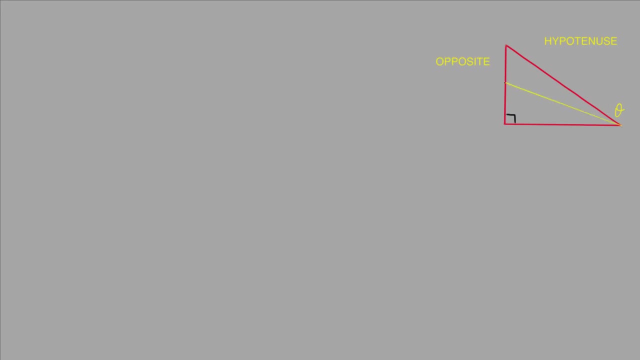 opposite side of the right triangle is always straight across or opposite of theta. If you draw a straight line from theta, you will intercept the opposite side. The adjacent side is the side that is adjacent to theta. That is not the hypotenuse. So let's see what. 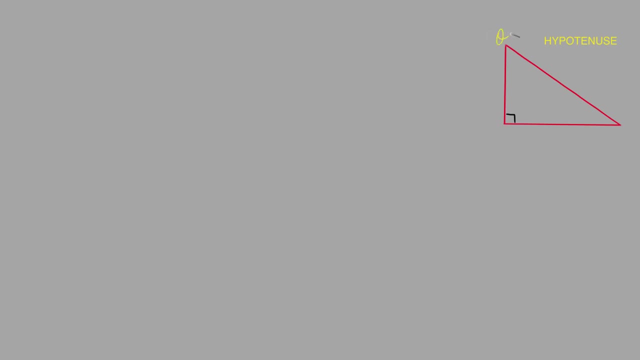 would happen if we drew a straight line from theta, happen if I put theta in this angle here. So that would make this side the opposite side, Because the opposite side must be opposite of theta, And that would make this side the adjacent side. The adjacent side has to be the side that is adjacent to theta, that is. 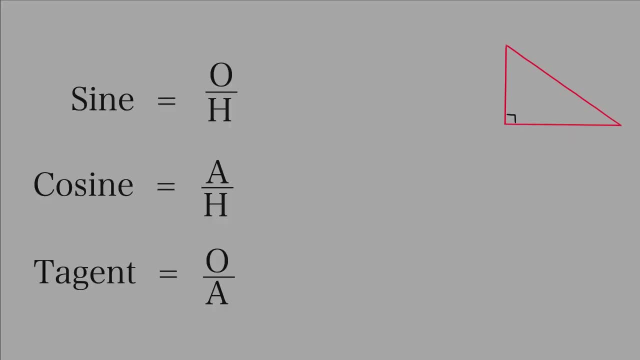 not the hypotenuse. Now that we've identified the sides of the triangle, let's look at how to use the three most basic formulas of trigonometry: Sine equals opposite over hypotenuse, Cosine equals adjacent over hypotenuse. And tangent. 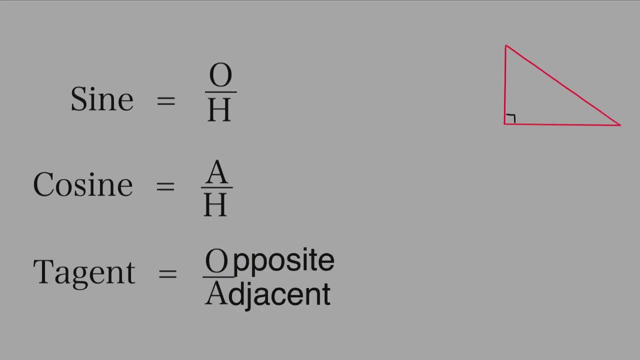 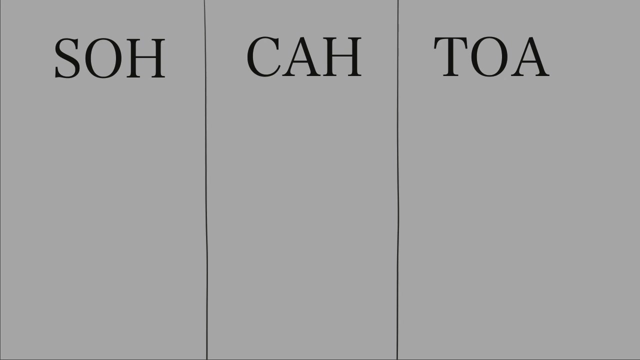 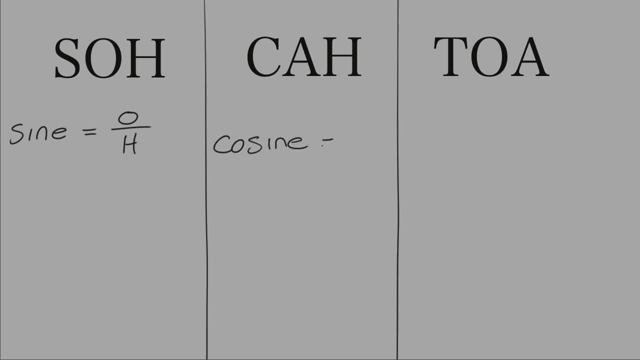 Means, cosine Is equal to adjacent over hypotenuse And toa means tangent Is equal to opposite over adjacent. These are the three main functions of trigonometry that we will mostly focus on in this video, But just so you are aware of it, there are also reciprocal functions. The reciprocal 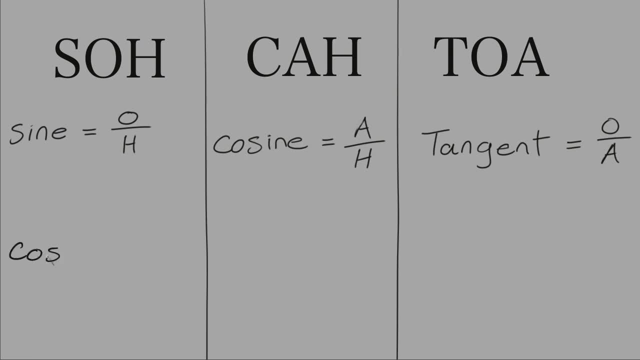 of Sine is cosecant. Cosecant is equal to hypotenuse over opposite. The reciprocal function of cosine is secant. Secant is equal to hypotenuse over adjacent, And the reciprocal of tangent is cotangent. Cotangent is equal to adjacent over opposite. So we'll try using the sine function to calculate. 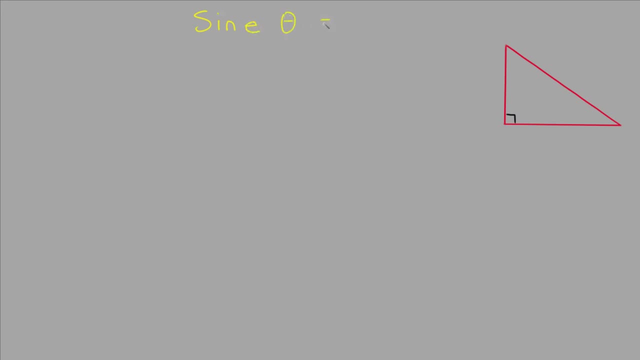 for the opposite side. So sine of theta equals opposite over hypotenuse. This is our hypotenuse side And this is our opposite side. Let's say we had an angle of 35. Our hypotenuse side is 17.43.. Opposite side is unknown, So we have. 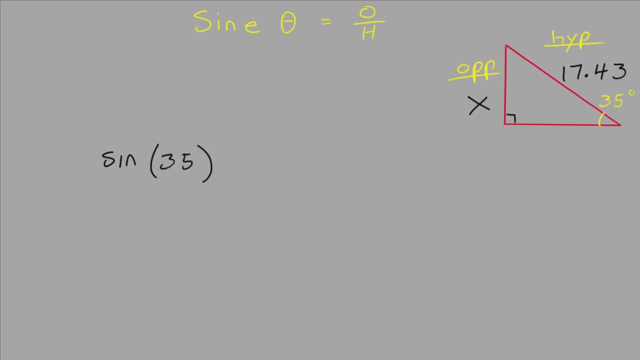 sine of 35,, which is equal to the opposite side, which is x over the hypotenuse, which is 17.43.. We'll want to isolate the variable of x by using inverse operations, So we'll multiply by 17.43. 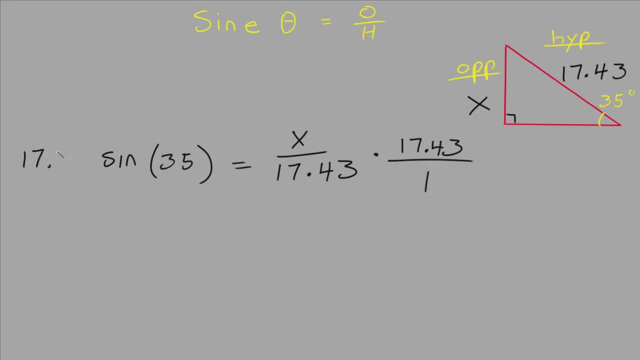 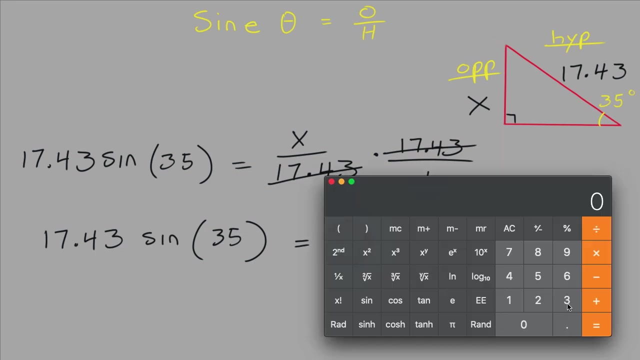 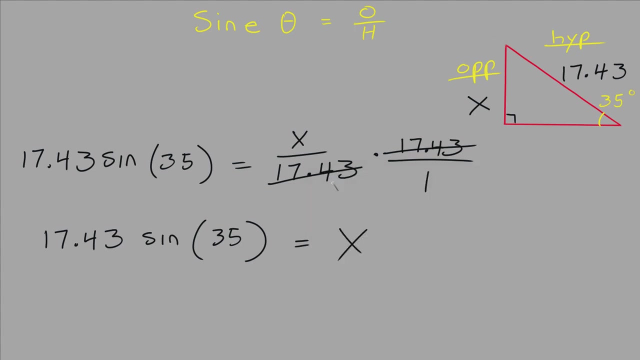 over 1.. We'll do the same thing on this side. These will be cancelled out And we're left with 17.43. sine of 35 equal to x. So x equals 9.99.. Just going to round that up to 10.. 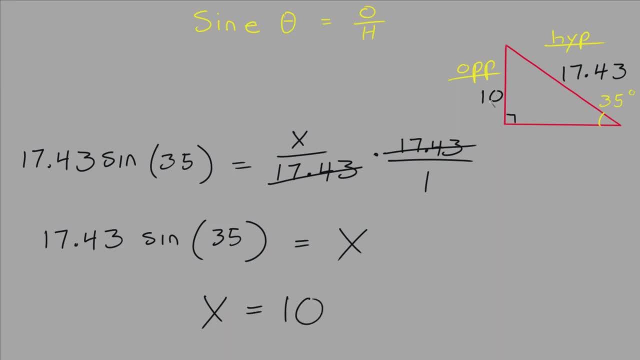 So we have solved the opposite side of the equation Using the sine function. let's use the sine function to solve for the hypotenuse side of our triangle. So we have: sine of 35 is equal to the opposite side, which is 10 over the hypotenuse. 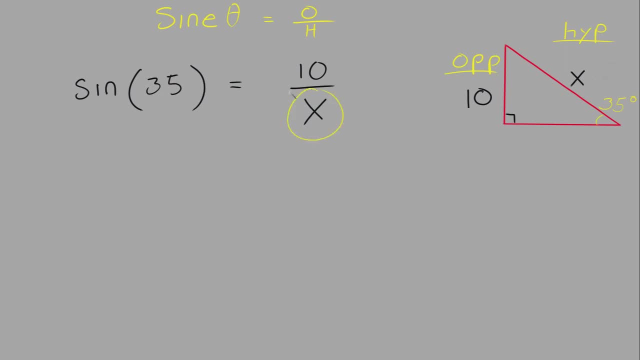 side, which is unknown, So we'll need to isolate the variable x. We'll cross, multiply: x multiplied by sine 35 is equal to 10.. We'll still need to isolate for the variable x, So we'll divide both sides by the sine of 35.. 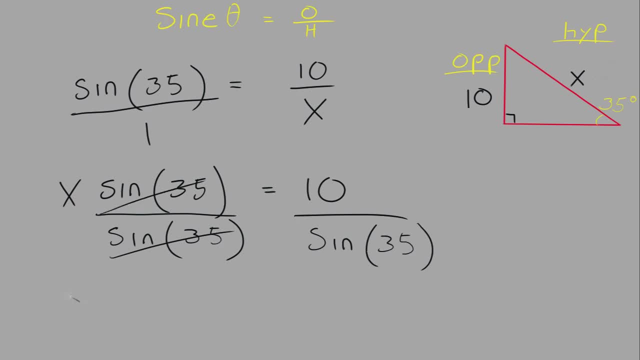 These will be cancelled out And it will leave us with x is equal to 10.. over the sine of 35.. x is equal to 17.43.. So we have solved for the hypotenuse side of our triangle: 17.43. 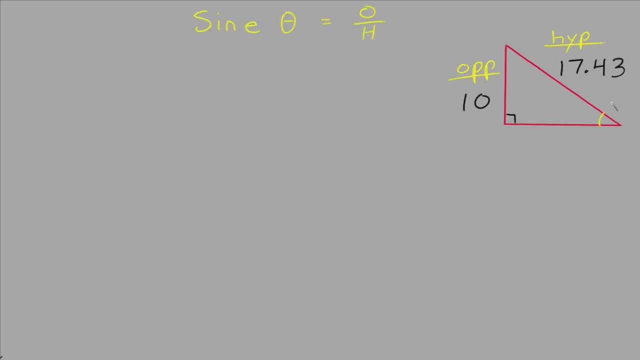 So this time we'll use the sine, We'll use 10.43,. This time we'll use the sine function to calculate for theta. So what we have is sine of theta is equal to the opposite side of 10 over 17.43.. 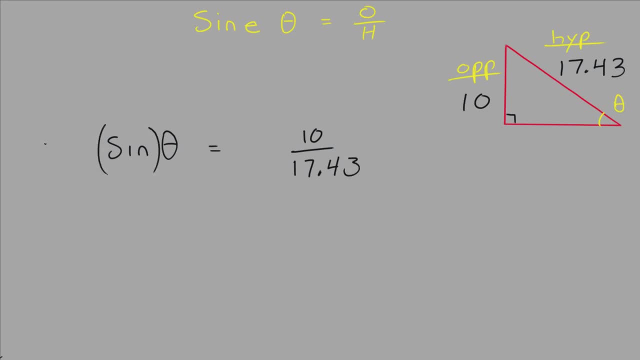 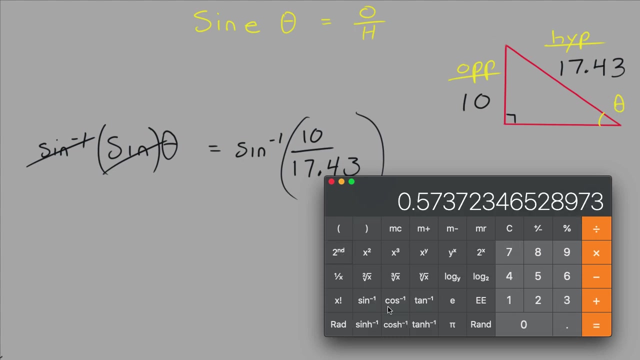 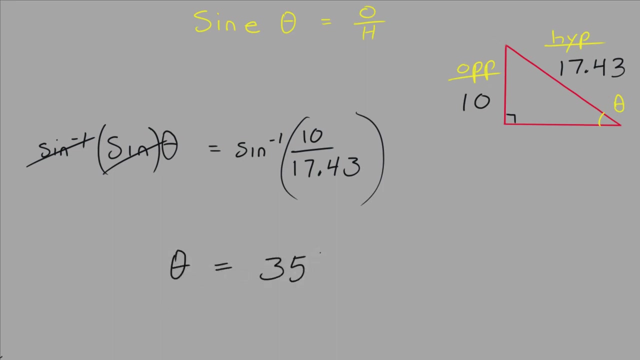 So to isolate theta we'll have to use the inverse function of sine, And we'll do that on both sides. So theta is equal to 35 degrees. So we have used the inverse of sine function to calculate the angle of 35 degrees. 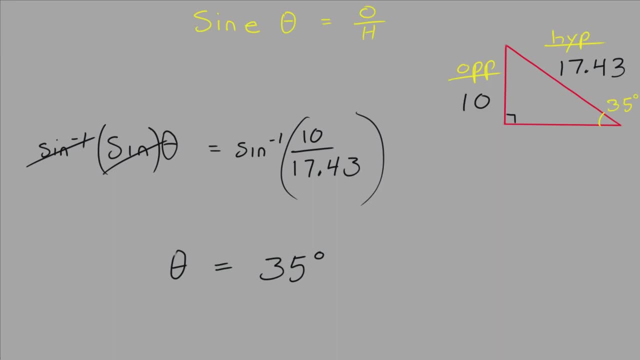 So we have used the sine function in 3 different ways. We solved for the hypotenuse, the opposite and the angle. Now we'll try using cosine of theta. Cosine of theta is equal to adjacent over hypotenuse. This is our hypotenuse side. 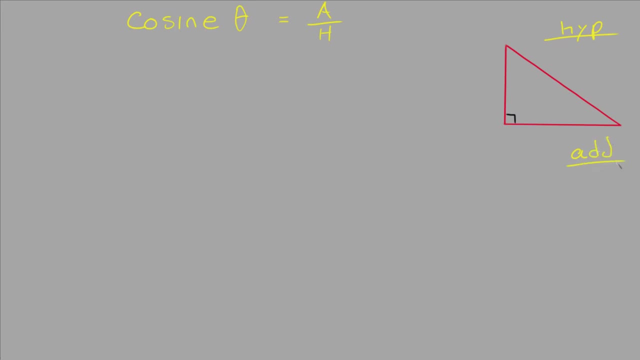 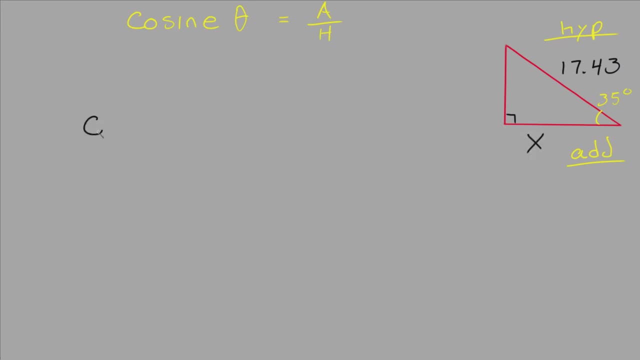 The adjacent side is unknown. So what we have is cosine of 35, and it's equal to the adjacent side, which is unknown, over the hypotenuse side, which is 17.43.. And to isolate the x variable we'll multiply by 17.43 on both sides. 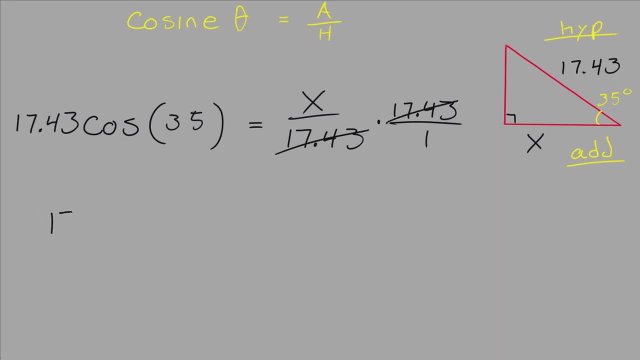 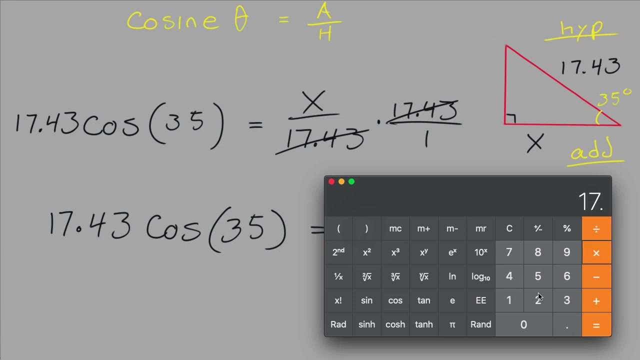 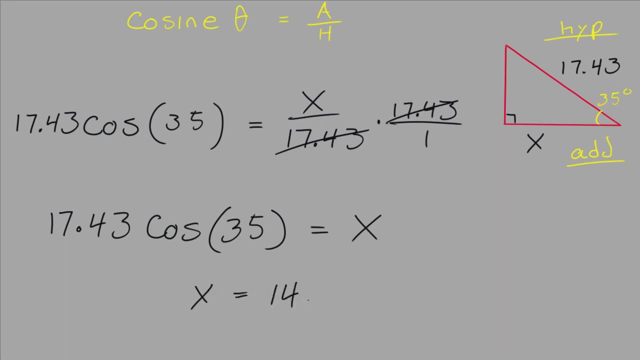 These will be cancelled out. So what we're left with is 17.43. cosine of 35 is equal to x, So x equals 14.28.. So we have solved for the adjacent side of our triangle. The adjacent side is 14.28.. 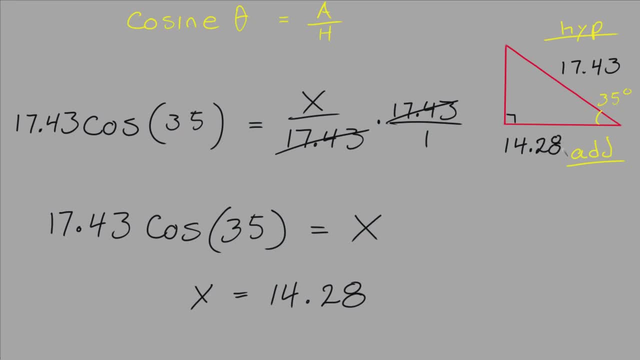 This time we'll try solving for the hypotenuse side of our triangle. So the hypotenuse side will be x and the adjacent side will be 14.28.. So what we have is cosine of 35 is equal to the adjacent side of 14.28 over x. 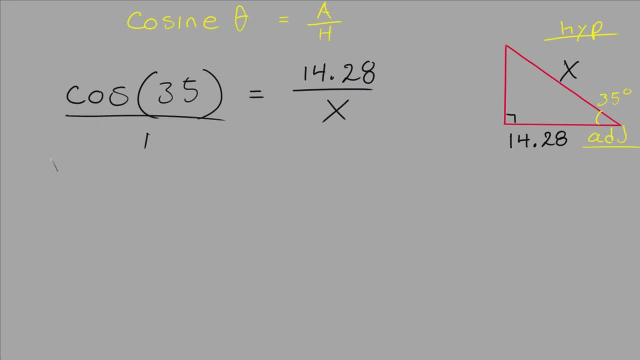 We'll isolate x, x by cross multiplying, and then we'll have x, cosine of 35, equal to 14.28.. We will divide by cosine of 35 on both sides. This will be cancelled out and we're left with: x is equal to 14.28 divided by cosine. 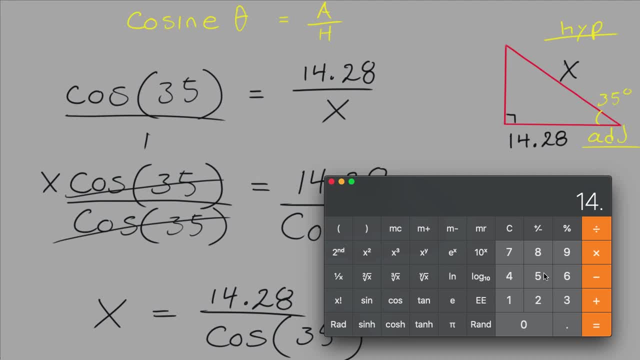 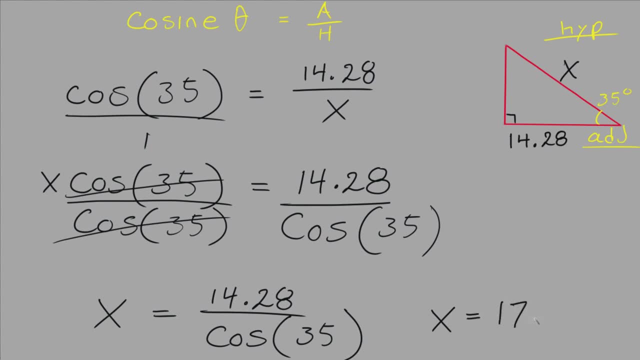 of 35, so x equals 17.43.. So we have solved for the hypotenuse side of our triangle. This time we'll use the cosine function to solve for theta. The hypotenuse is 17.43 and the adjacent is 14.28. 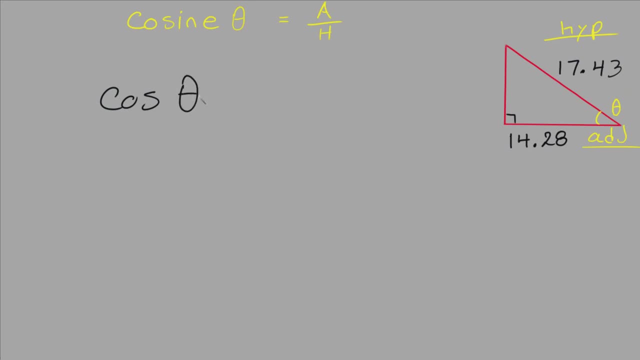 So we have cosine. theta is equal to the adjacent of 14.28 over the hypotenuse of 17.43.. To isolate theta we will multiply by the inverse function. This is the inverse function of cosine on both sides. These will cancel out and what you'll have left is theta is equal to inverse of cosine. 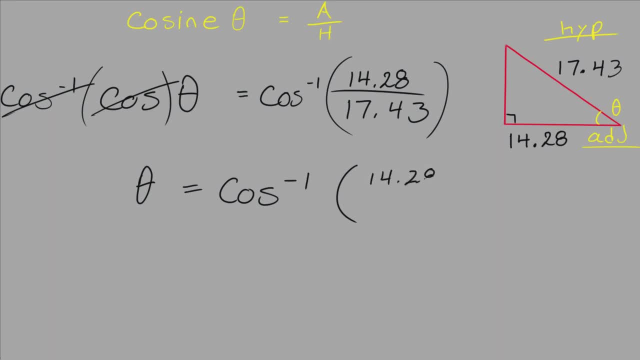 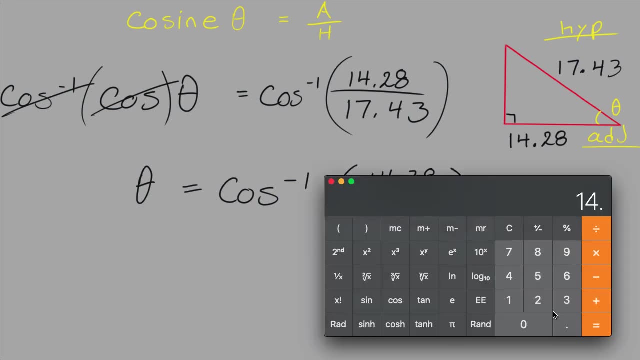 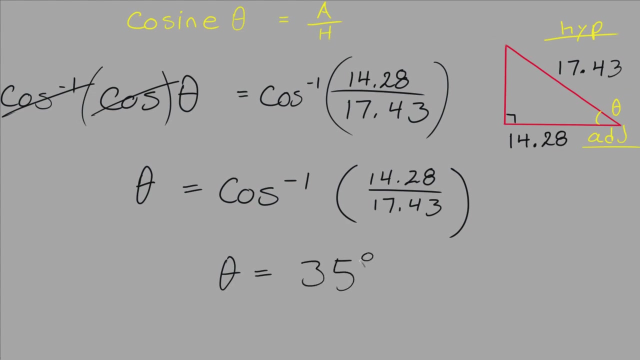 14.28 divided by 17.43.. And I'll just round that up. so theta is equal to 35 degrees. So using the inverse of cosine function, we have solved for the angle of our triangle 35 degrees. So we'll be using the tangent function for the next three examples. 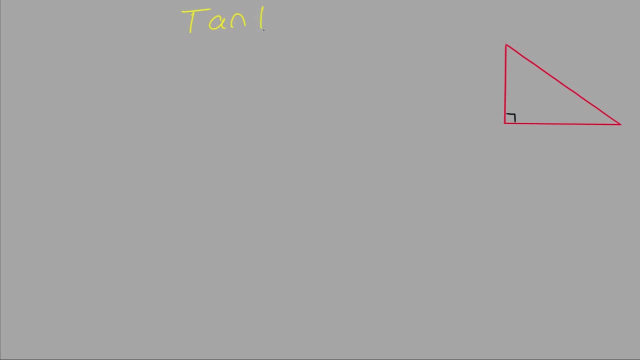 I'll explain that later Now. in the next video I'll explain how to solve for the tangent of theta. In the next video I'll explain how to solve for the tangent of theta. tan of theta is equal to opposite over adjacent. 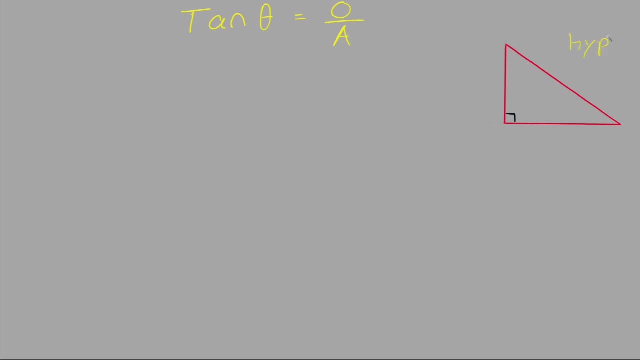 This is the hypotenuse side. This is the opposite side. The angle is still going to be 35 degrees and this is the adjacent side. The adjacent side is 14.28.. The opposite side is unknown, so we'll try solving for the opposite side. 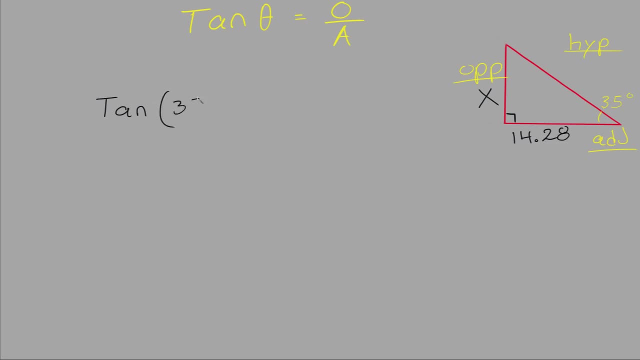 So we have tan of 35, and it's equal to the opposite side of x over the adjacent side of 14.28.. To isolate for the variable x we'll need to multiply by 14.28. On both sides Okay. 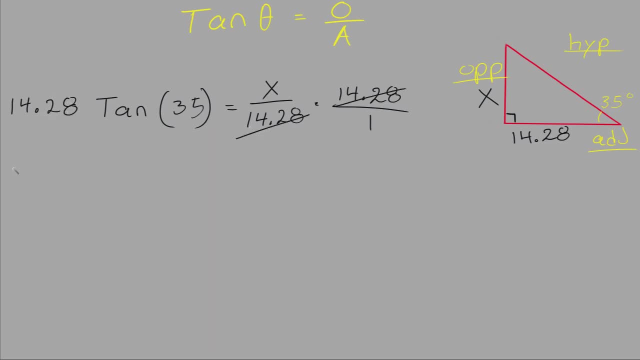 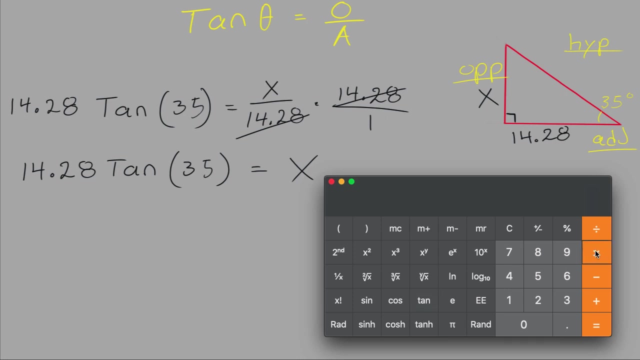 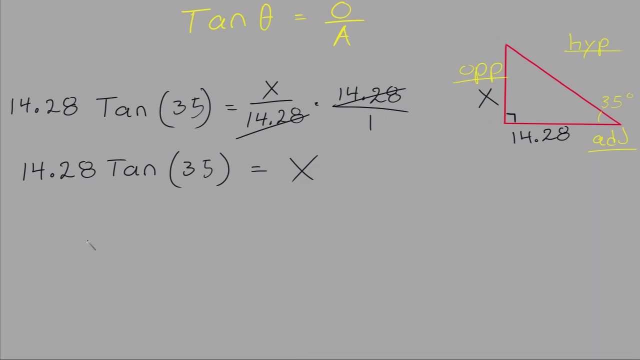 These will be cancelled out and we're left with 14.28. tan of 35 is equal to x, So x equals 10.. So we have solved for the opposite side Using the tan function, So now we'll use tan to solve for the adjacent side. 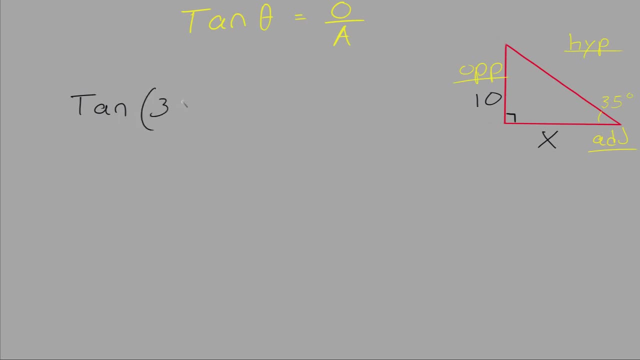 So we have: tan of 35 is equal to opposite side of 10 over the adjacent side which is x. So we need to isolate the variable x. So we'll cross, multiply And we'll have x And we'll have x multiplied by tan, 35 equals to 10.. 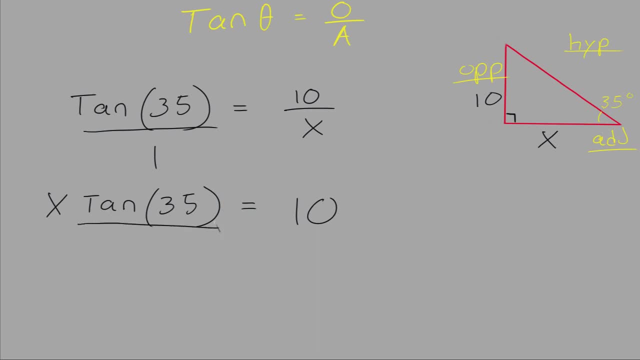 We still need to isolate for x, So we'll divide both sides by tan 35. These will be cancelled out And we're left with x is equal. Can we solve for this? Can we solve for x If we can't solve it? 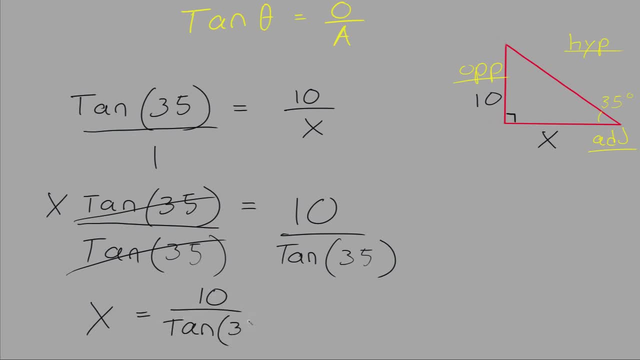 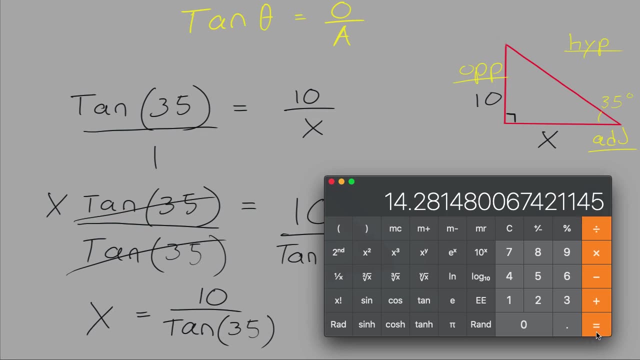 Just take x and downsize it. So let's take this. Let's take this: K is equal to 14.28.. We'll make a duplicated capital X, And now this is 15.25.. So we'll make a common capital X.